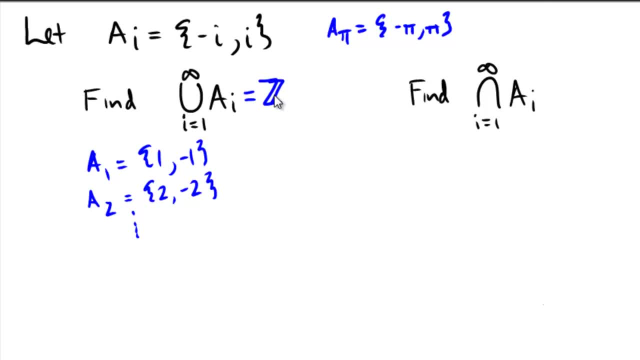 Well, you're going to get almost all of z right. z is almost completely in there, all of the integers and all of the negative integers, but not the number zero. So the correct answer to this is z, And z is a number of integers minused by 0, not including 0.. 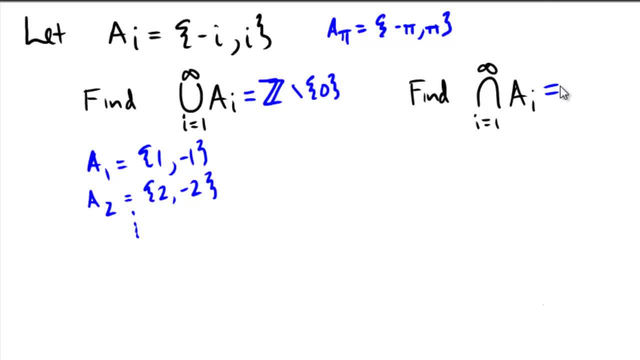 How about the intersection? The intersection's even easier, it turns out. We already wrote out two of the sets over here, remember a1 and a2.. What numbers do those sets have in common? Well, 1 and negative. 1 are in the top one. 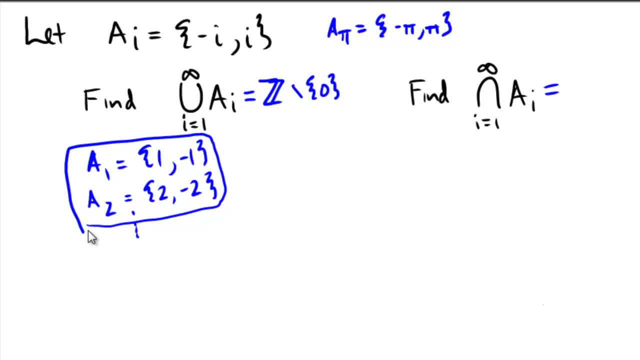 2 and negative 2 are in the bottom one. There is nothing in common, So we don't even need to look at the other ones. The first two sets don't have any common numbers, even have anything in common, So the answer here is going to be a null set. There is nothing in. 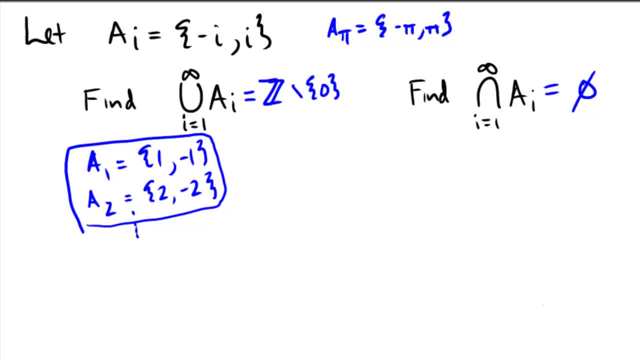 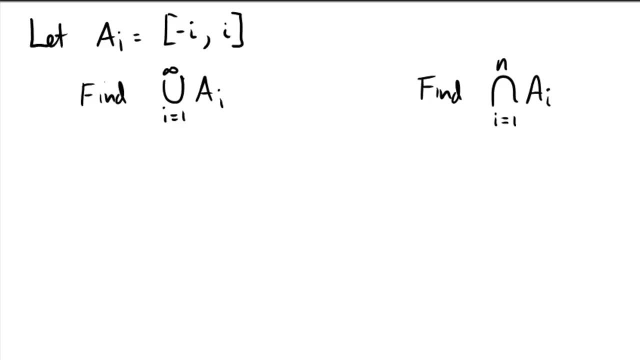 common when you intersect. all of these sets down. So why don't you pause the video and try one here on your own? I have here the a sub i's being the closed intervals from negative i to i. So pause the video and see if you can find these unions and intersections. 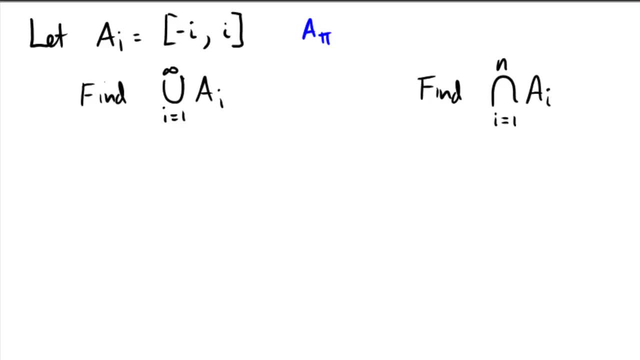 Okay, to begin with I'm going to do one example up here so we can kind of see what it looks like. a sub pi would be the interval from negative pi to pi or the set of x, such that negative pi is less than or equal to x is less than or equal to pi. Now that negative pi is a little bit unclear, Here we go. 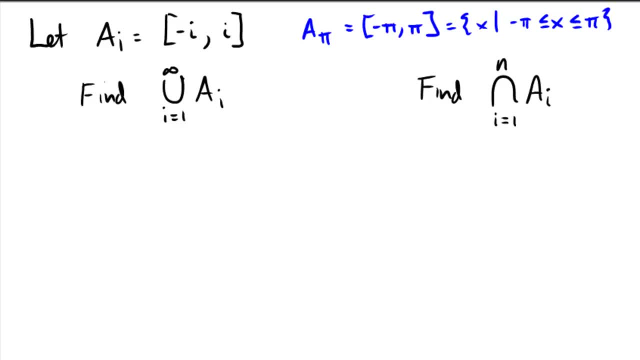 negative pi. Okay, so come over here again and let's kind of approach it the same way we did last time. We're now indexing over natural numbers one, two, three, four, five. So a sub one is equal to the closed interval from negative one to one. Now the order is important because 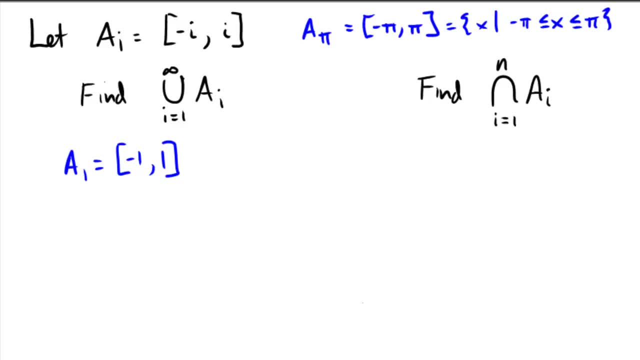 we want to start at the lower number and end at the higher number. So negative one to one, a sub two is going to look like the closed interval from negative two to two, And that goes on and on and on. So what's happening here is it looks like we're going from. 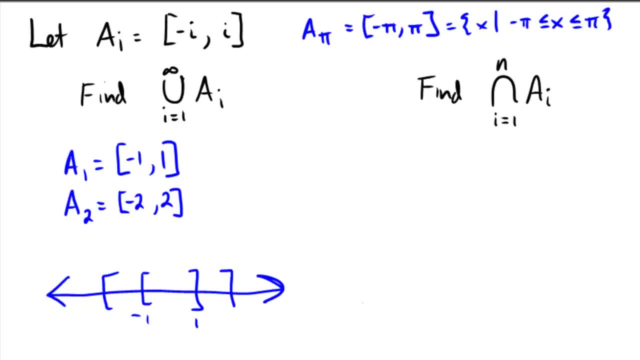 negative one to one, and then negative two to two, and then dot, dot dot and dot dot dot. So this is going to be the closed interval from negative one to one. These intervals are constantly expanding, right, they're going to get larger and larger and larger.